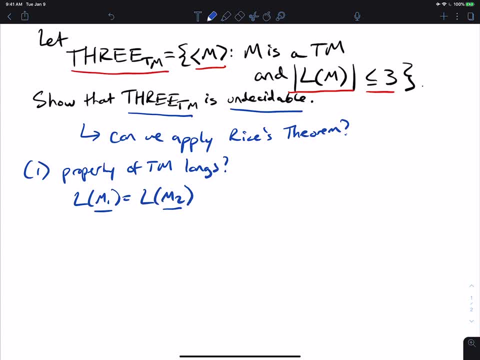 Well, let's think about it. Well, if they have the same language, well then they have the same number of strings in the language. So that implies that either both M1 and M2 are in 3TM, Either they both have at least four strings, or M1 and M2 are not in. 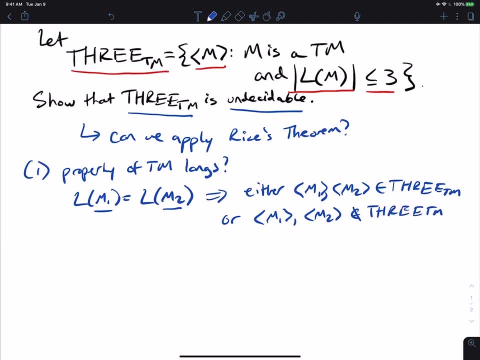 3TM, because if they are the same language, then they either both have at most three strings or at least four strings. So what we conclude from this is that this is indeed a property of Turing machine languages. Now, the other thing that students sometimes forget is 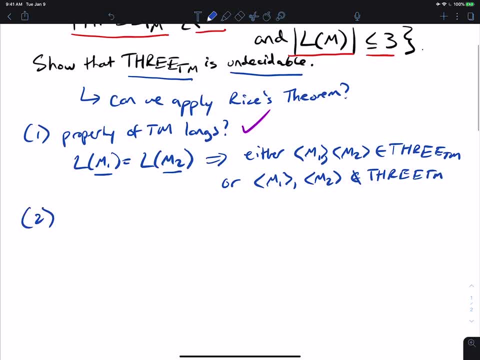 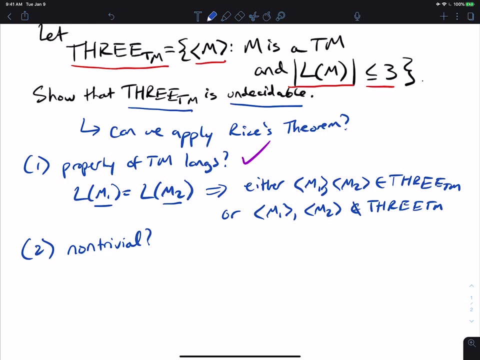 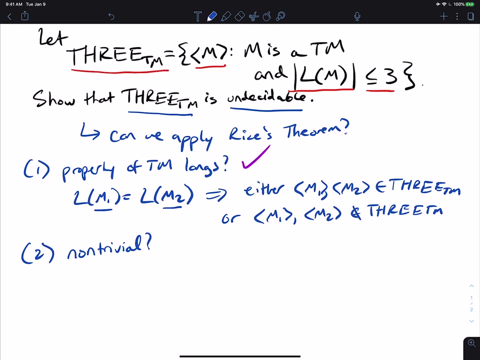 is this a non-trivial property? So is this property. I could spell it non-trivial. So that means, is there a Turing machine inside 3TM And is there a Turing machine that's outside 3TM? Well, can we find a Turing machine that accepts more than three strings, So at least four strings? 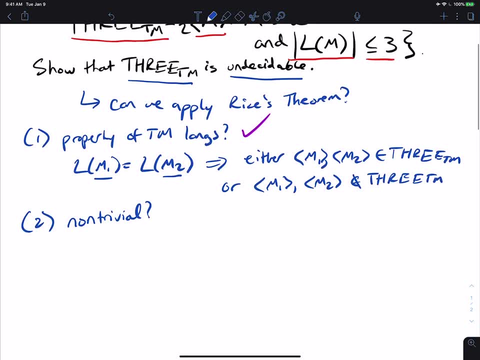 Well, a really easy example is: the Turing machine accepts everything. So let's let M1 be a Turing machine that accepts everything, So every single string it accepts. Well then, this implies that M1 is not in 3TM, Because, well, if it accepts everything, well, it accepts more than three strings. 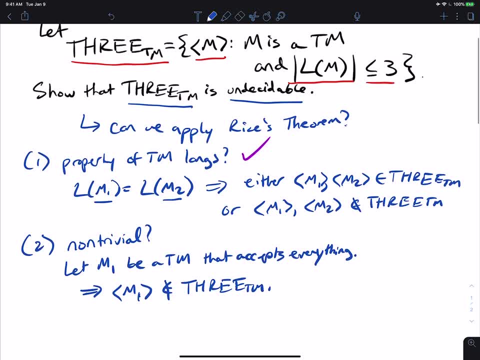 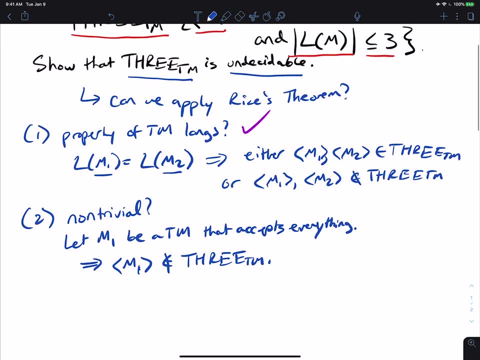 which therefore is not in 3TM. Well, can we find an example of a machine that is in 3TM, So it accepts at most three strings? Well, what we can do here is let M2 be a Turing machine that rejects everything, just says no, I don't accept it. 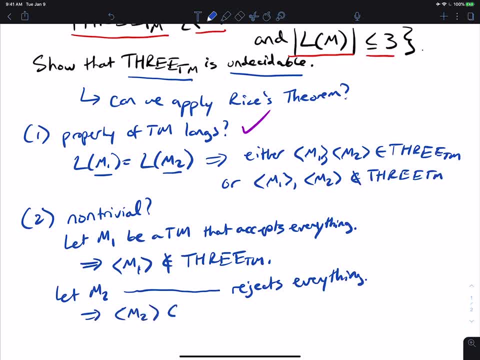 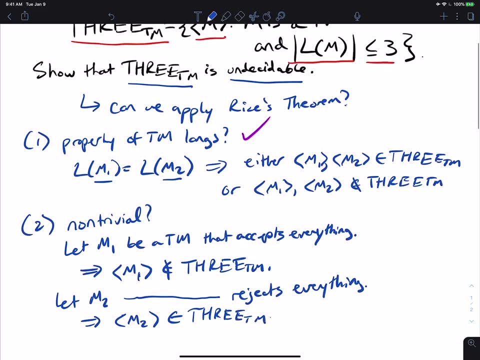 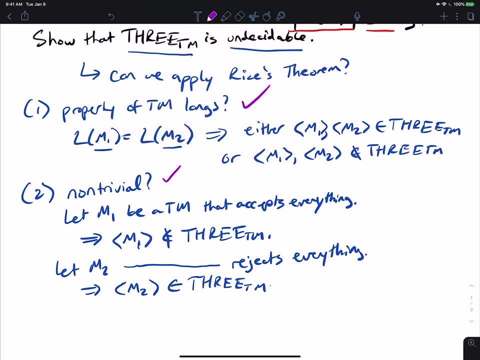 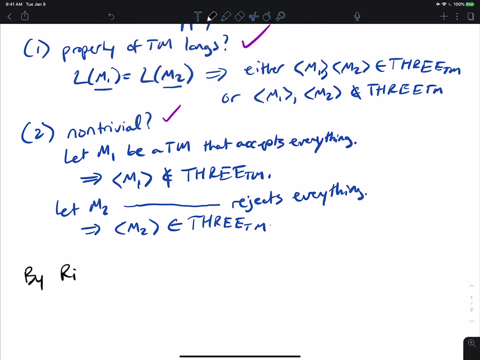 Well, that implies that M2 is in 3TM because it accepts zero strings which, as far as I can tell, is at most 3.. So we can conclude from this that this property is non-trivial. So the most important part, right here, by Rice's theorem, it's a non-trivial property.